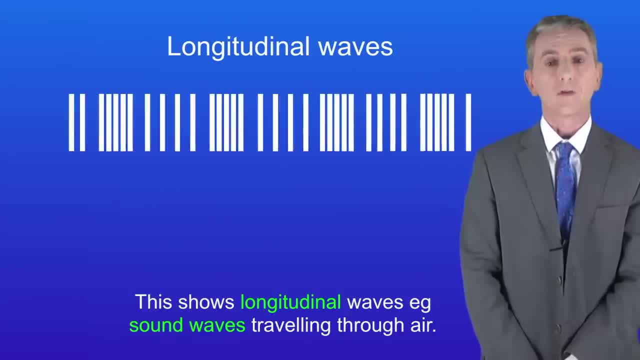 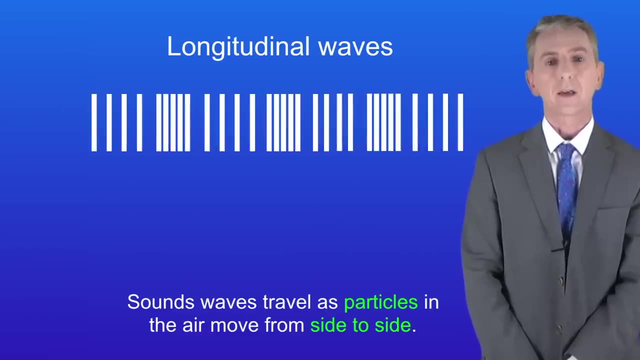 Okay, we're going to look now at the second category of waves. These are longitudinal waves, and I'm showing you a longitudinal wave here Now. a good example of a longitudinal wave are sound waves travelling through air. Sound waves travel as particles in the air move from side to side. So here I'm showing you. 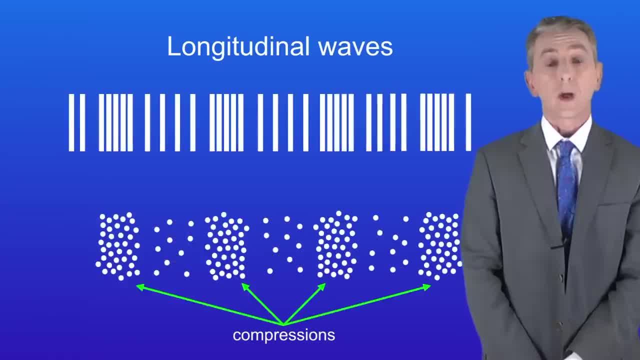 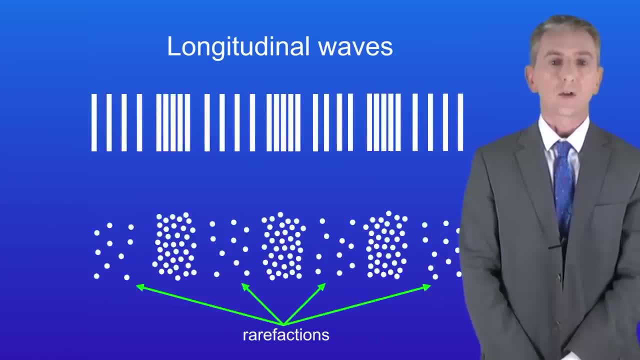 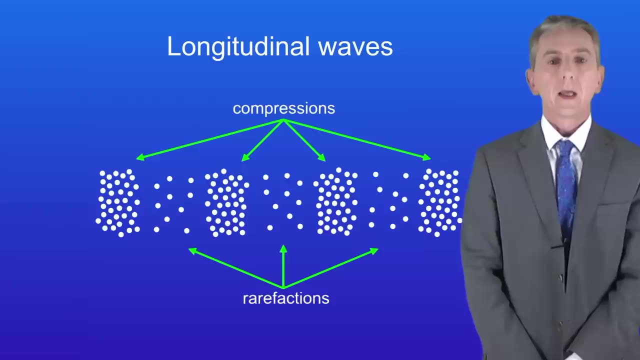 the air particles. You can see that we've got regions where the air particles are very close together. Scientists call these regions compressions. In between the compressions, we've got regions where the air particles are spaced out, and scientists call these regions rarefactions. 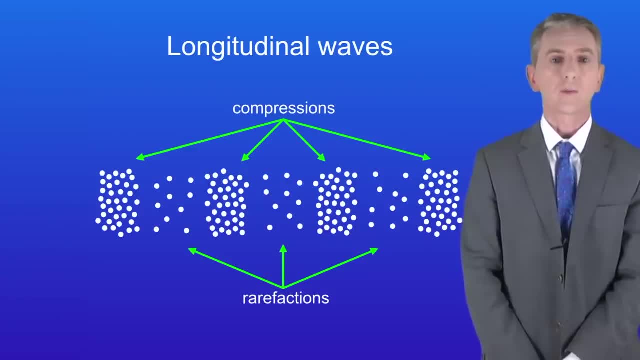 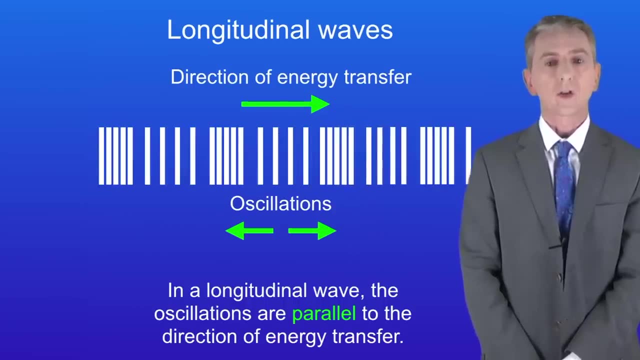 Here I've paused the wave So you can see the compressions and rarefactions more clearly Now. unlike with transverse waves, the key feature of a longitudinal wave is that the oscillations are parallel to the direction of energy transfer, and we can see that here. 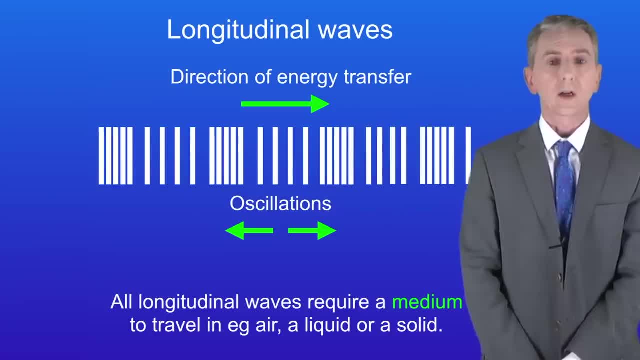 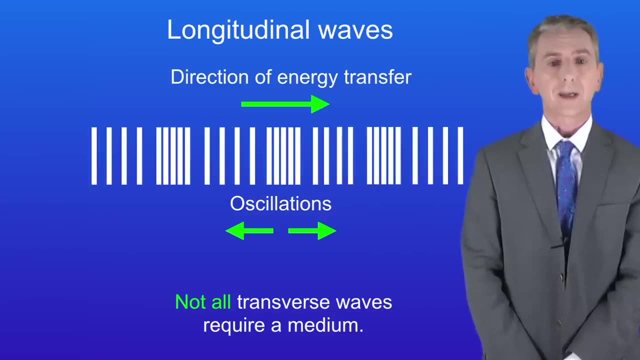 Now there is one other key difference between transverse and longitudinal waves. All longitudinal waves require a medium to travel in, For example, air, a liquid or a solid. In contrast, not all transverse waves require a medium, And we're going to look at some of those in later videos. 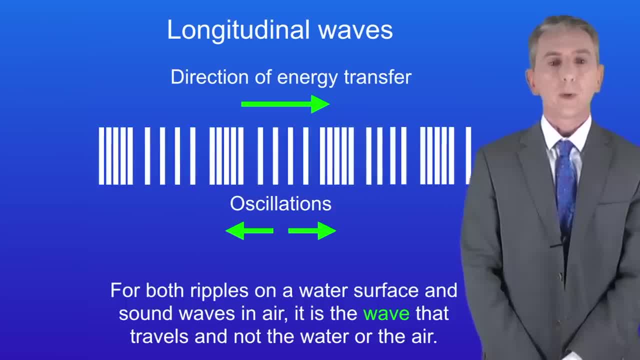 Now there's one really important fact that you need to learn about waves, For both ripples on a water surface and sound waves in air, it's the wave that travels and not the water or the air. We can see that using a slinky. This shows transverse waves and this represents 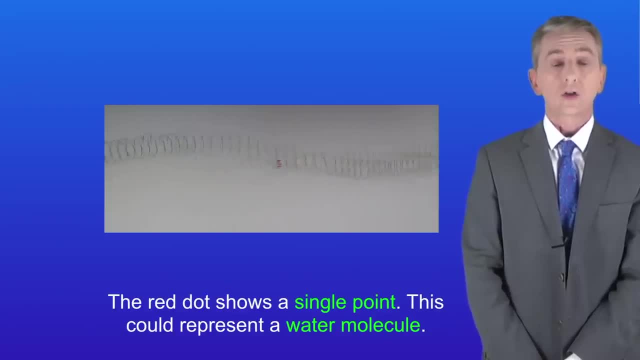 ripples on the surface of water. The red dot shows a single point and this could represent a water molecule. As you can see, when the waves travel through air, they're not always transparent. It's just a single point And this could represent a water molecule, As. 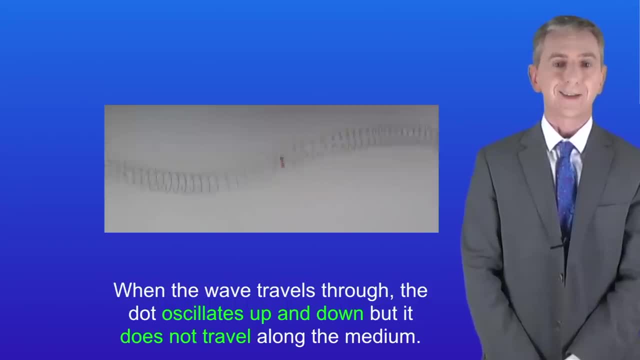 you can see, when the waves travel through air, they're not always transparent. This the wave travels through the dot, oscillates up and down, but it does not travel along the medium. Now I'm sending longitudinal waves along the slinky. This represents sound waves travelling. 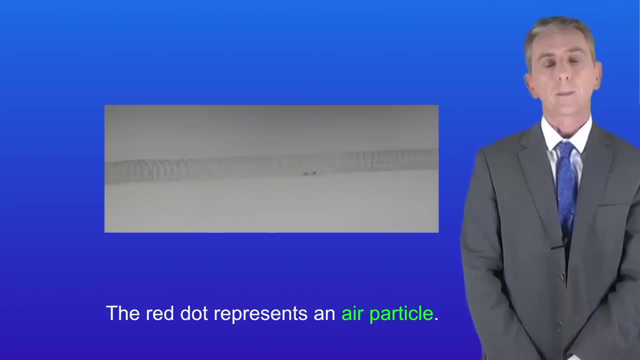 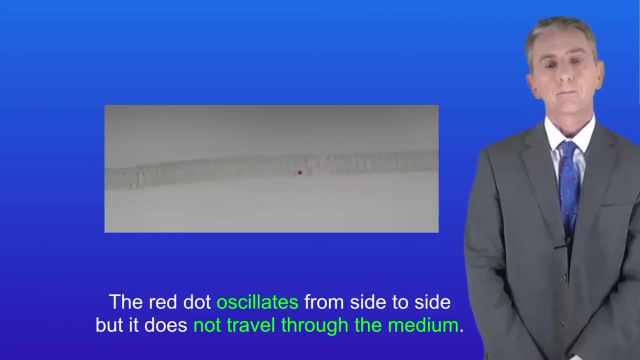 through air and the red dot represents an air particle. As you can see, the red dot oscillates from side to side but, again, it does not travel through the medium. Remember: you'll find plenty of questions on transverse and longitudinal waves in my 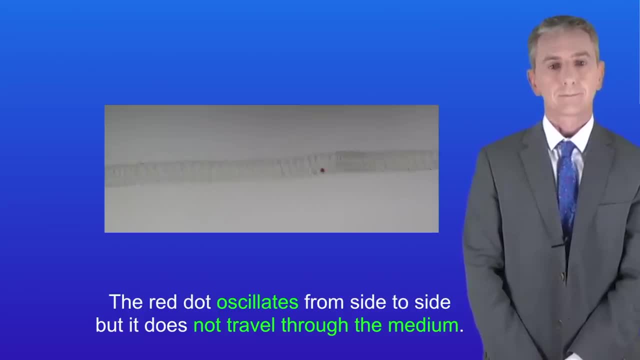 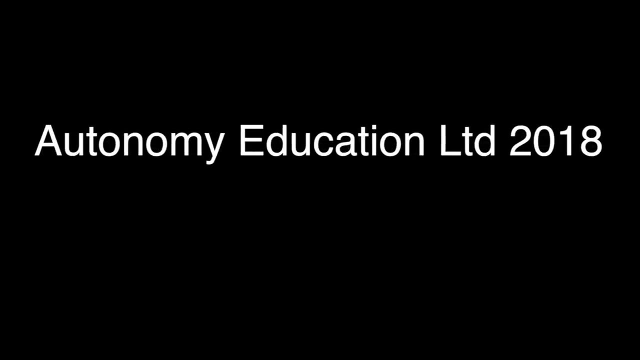 vision workbook and you can get that by clicking on the link above.